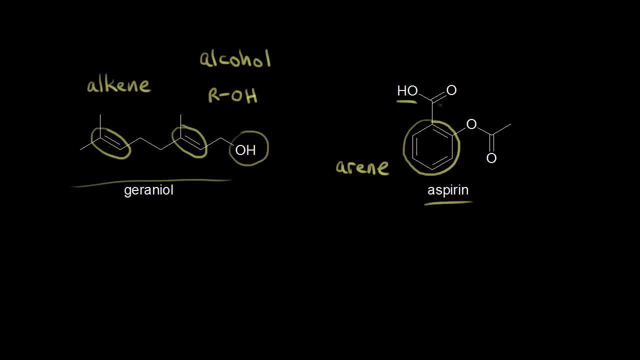 present in aspirin. What about this one up here? We have an OH and the oxygen is directly bonded to a carbonyl. So let's go ahead and write that out. We have an OH where the oxygen is directly bonded to a carbon, double bonded to an oxygen, and then we have 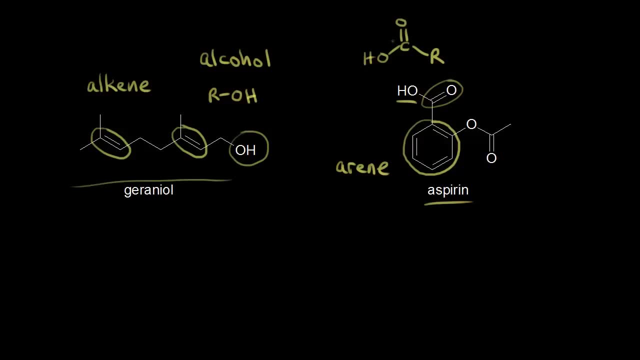 the rest of the molecule. So hopefully you recognize this as being a carboxylic acid. So let me go ahead and write that out here. So this is a carboxylic acid. Alright, our next functional group. We have an oxygen, and then oxygen is directly. 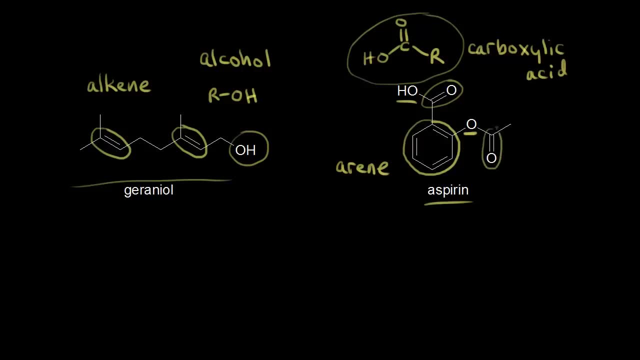 bonded to a carbonyl. So here's a carbon double bonded to an oxygen. So let's write this out: We have an oxygen directly bonded to a carbonyl, And then for this oxygen we'd have the rest of the molecule. So that's all of this stuff over here, And then 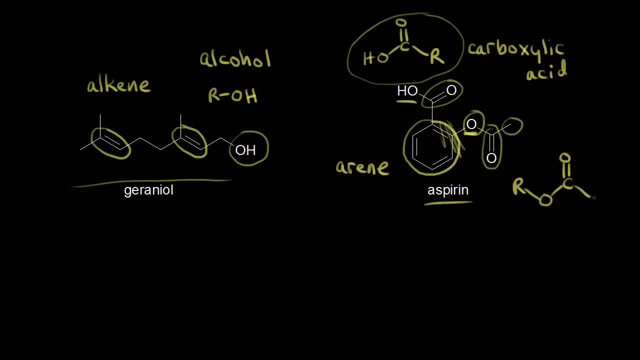 on the other side of the carbonyl we have another R group, So I'll go ahead and write that in. So that is an ester ROC double bond. O R is an ester, So there's an ester functional group. 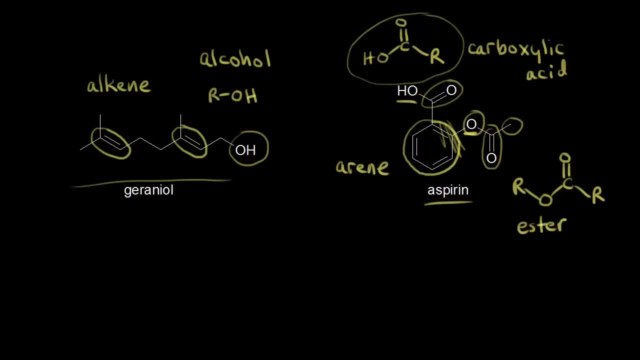 present in the aspirin molecule. Let's look at some of the common mistakes that students make. One of them is students will say a carboxylic acid is an alcohol, So let me write out here a carboxylic acid, so we can talk about that. 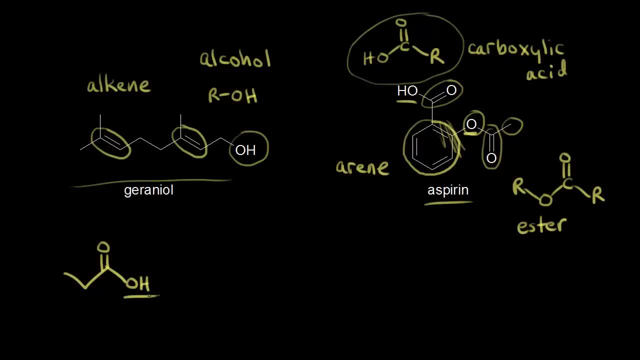 So sometimes the students will look at that and say, oh well, I see an OH and then I see the rest of the molecule. So isn't that an alcohol? But since this oxygen is right next to this carbonyl, this is a carboxylic acid. So this is an example of a carboxylic. 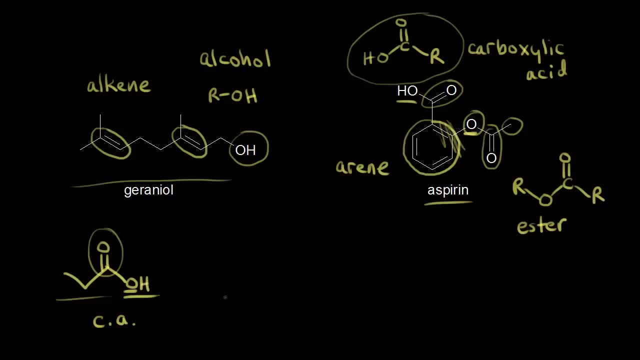 acid. If we moved the OH further away from the carbonyl, Let's go ahead and draw one out like that. So here is our carbonyl, And now the OH is moved further away. Now we do have an alcohol, Now we have an OH and then the rest of the 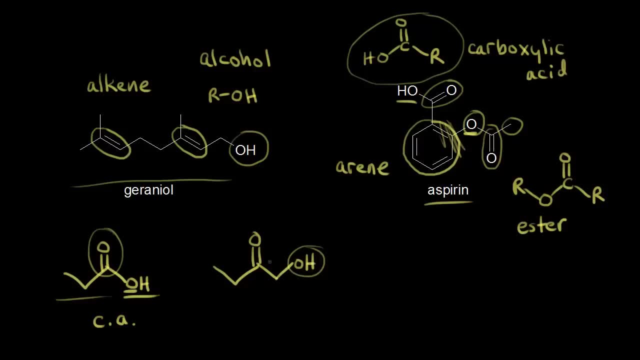 molecule. So this would be. let me go ahead and use a different color here. So now we are talking about an alcohol. So this is an alcohol, And what would this one be? We have a carbonyl and then we have an R group on one side. 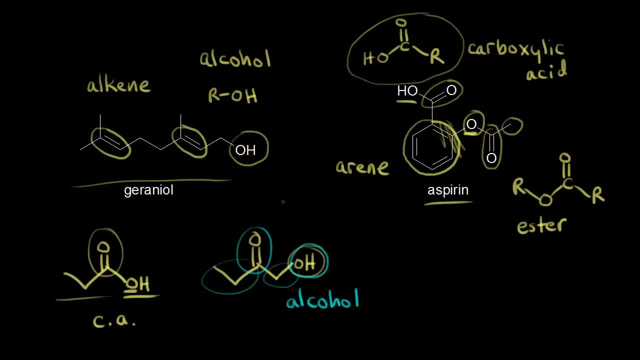 and an R group on the other side. That is a ketone. Let me draw this out. So when you have a carbonyl and an R group on one side and an R group on the other side, They could be the same R group. They could be a. 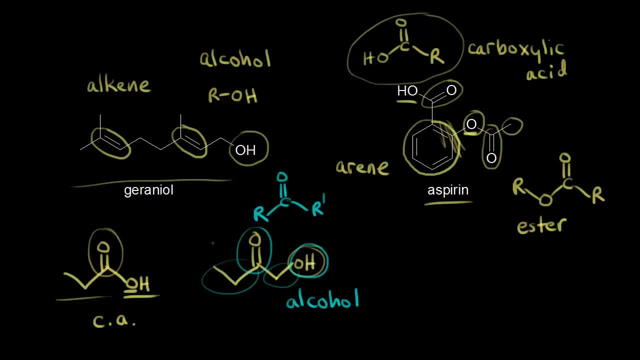 different R group. Sometimes you'll see like R prime drawn for that. So this is a ketone. So now we have a ketone and an alcohol, So two functional groups present in the same compound. So hopefully you can see the difference between this compound. 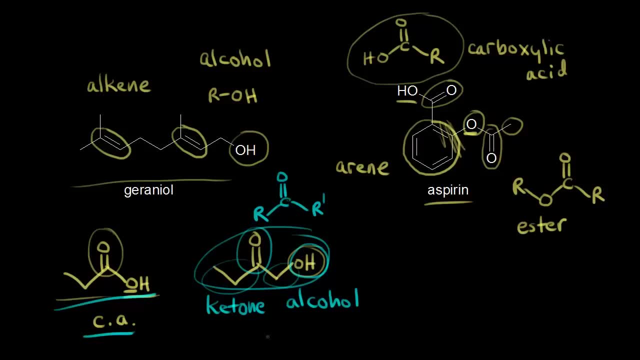 and this compound. This one is a carboxylic acid and this one is a ketone and an alcohol. Alright. another common mistake that I've seen a lot is on this functional group right here on aspirin. Students will look at this oxygen here and say, okay, I have an oxygen and I have. 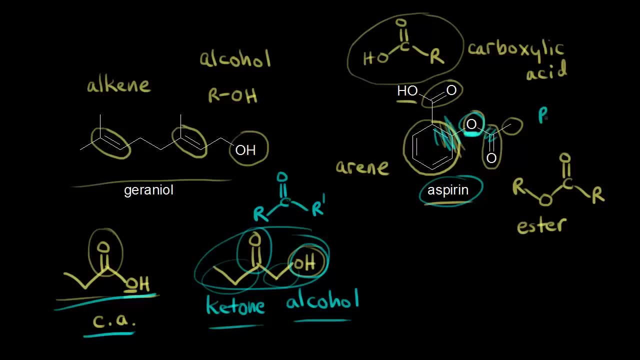 an R group on one side and I have an R group on the other side. So an R group on one side of the oxygen and an R group on the other side of the oxygen- Isn't that an ether? Well, this is R-O-R. 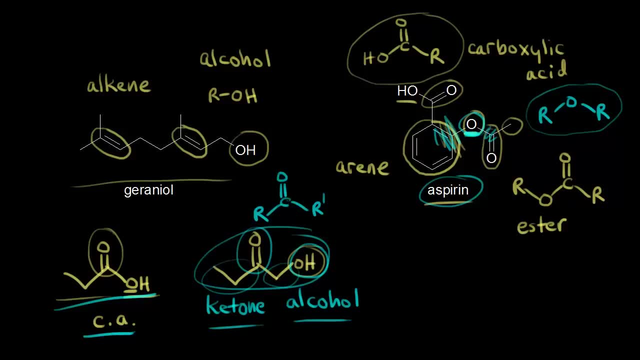 would represent an ether. However, we have this carbonyl here, So this carbonyl right next to this oxygen is what makes this an ester. How can we turn that into an ether? Let me go ahead and redraw this molecule here. 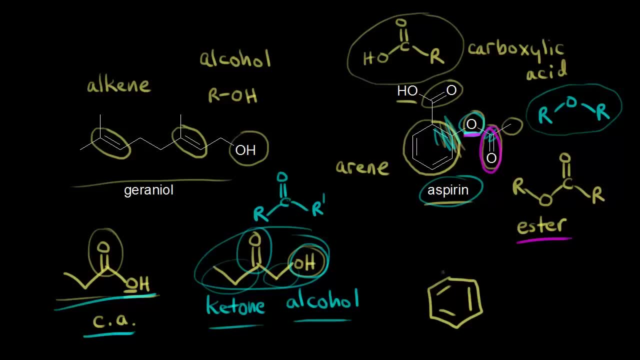 So I'll first put in our ring. So I drew the double bonds a little bit differently from how I drew it up here, but it doesn't really matter- And then I'll put in our carboxylic acid up here, And now, when I draw in this oxygen I'm going to take out the carbonyl. 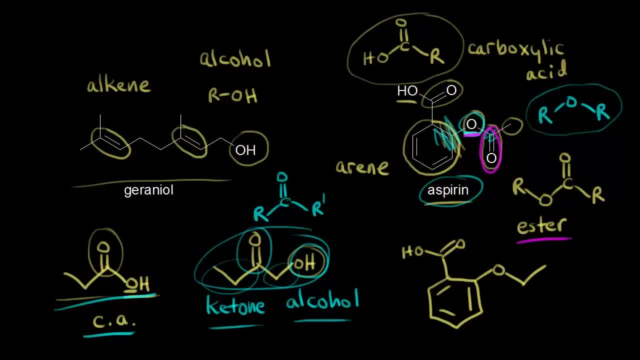 So now the carbonyl is gone And now we do have an ether. So this actually is an ether. now We have an oxygen, We have an R group on one side and we have the rest of the molecule over here on the other side. So now this is an ether. 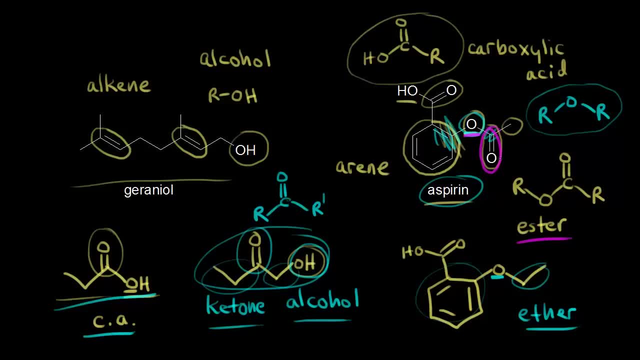 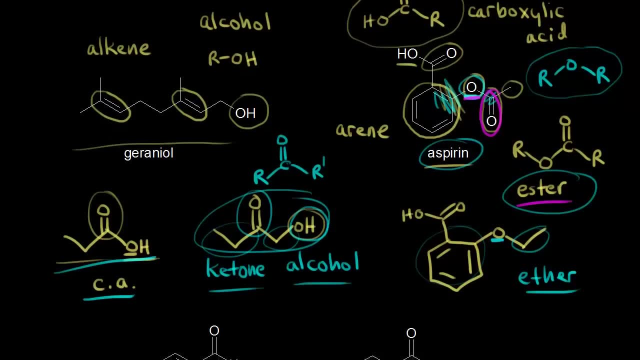 So hopefully you see the difference there. Look for the carbonyl right next to the oxygen. That makes it an ester. Alright, some more common mistakes that students make is they mix up these two functional groups. So let's look at the functional groups in these two molecules. here We start with. 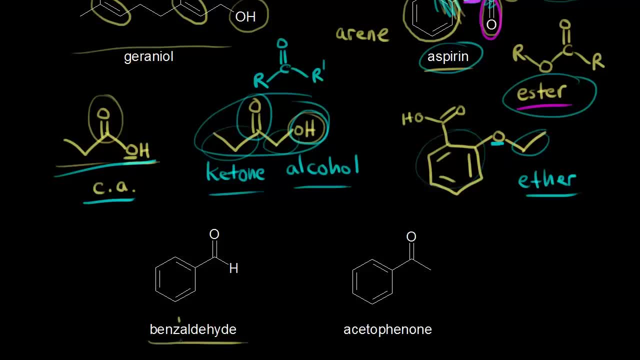 benzaldehyde, And the name is a dead giveaway as to the functional group. We're talking about an aldehyde here. So first we have our aromatic ring, our arine, And then we have an aldehyde. We have a carbonyl. 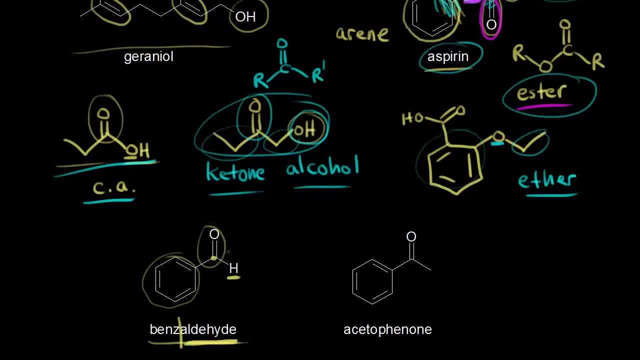 and we have a hydrogen that's directly bonded to the carbonyl carbon. So we have an R group and then we have a carbonyl, and then we have a hydrogen directly bonded to our carbonyl carbon. That is an aldehyde. If we took off that hydrogen, 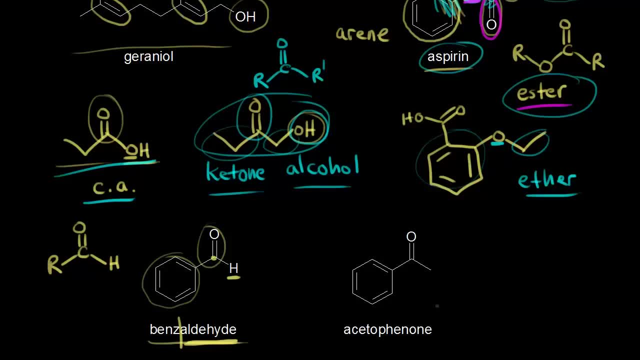 and we put a CH3 instead. that would be the compound on the right. So now we have a CH3 directly bonded to this carbonyl carbon. So now we have an R group on one side a carbonyl and then another R group, So we have R. 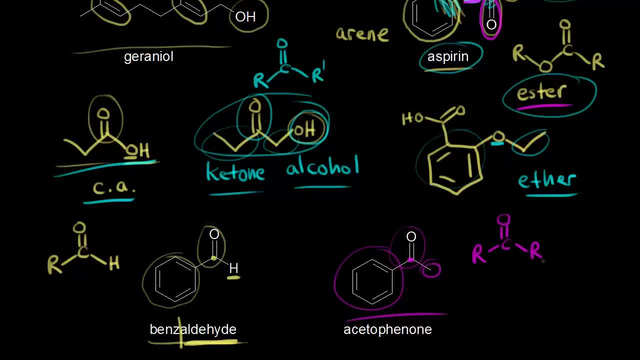 C, double bond O, R, And that is a ketone And you can tell by the ending of our name here that we have a ketone present in this compound. So again, this difference is subtle, but it's important And a lot of students 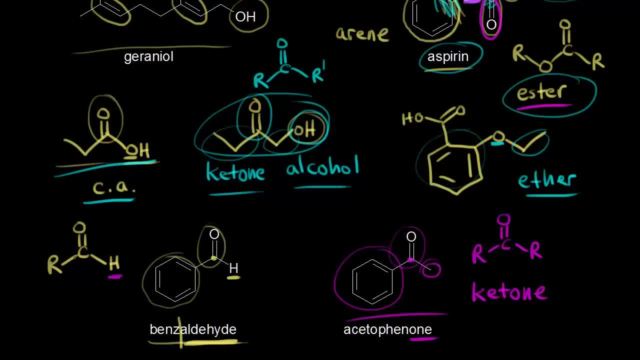 mess this up. An aldehyde has a hydrogen directly bonded to this carbonyl carbon. But if there's no hydrogen, we're talking about a ketone here. So R C, double bond, O R is a ketone. Finally, let's look at one giant. 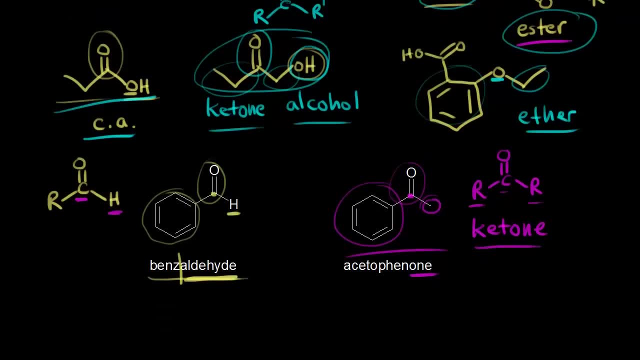 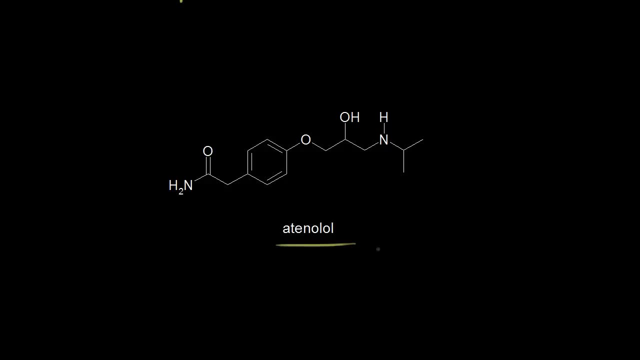 compound with lots of different functional groups, And let's see if we can identify all the functional groups present in this molecule. This molecule is called atenolol. This is a beta blocker, So this is a heart medication. Alright, let's look for some functional. 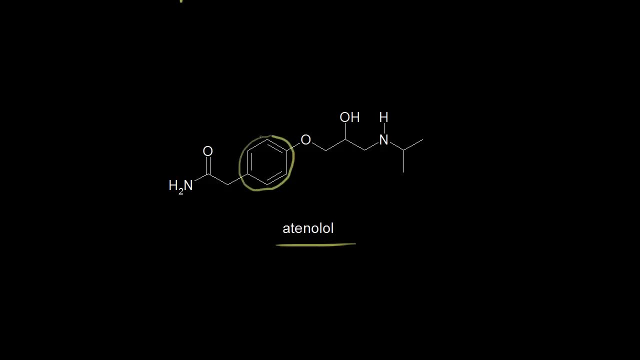 groups we've seen before. Here is that aromatic ring. So we know that an arene is present in atenolol, So let me go ahead and write this in here. Next, we have an oxygen And there's an R group on one side of the oxygen. 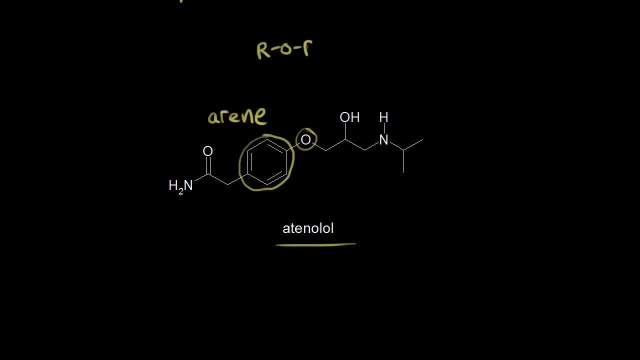 and an R group on the other side of the oxygen. So R O? R. we know that's an ether, So there's an ether present in this compound. Next we have an OH and then the rest of the molecule. So ROH would be an alcohol. 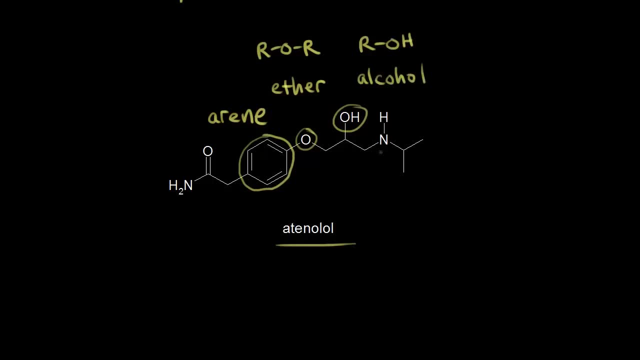 So there's an alcohol present, Alright. next we have a nitrogen with a lone pair of electrons. There's an R group on one side, There's an R group on the other side. So this is an amine. So we have an amine. And finally, over. 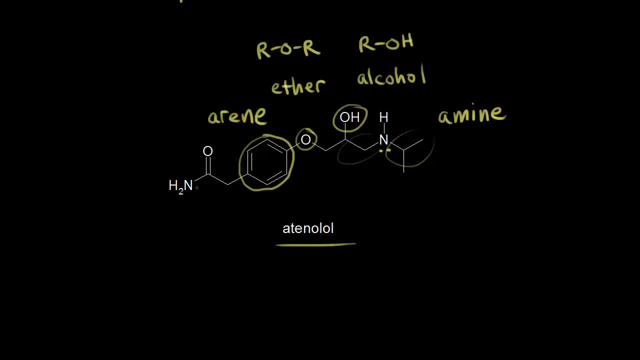 here on the left, So this is one that is messed up a lot. We do have a nitrogen with a lone pair of electrons on it, So it's tempting to say we have an amine here, But this nitrogen is right next to a carbonyl, So it's not. 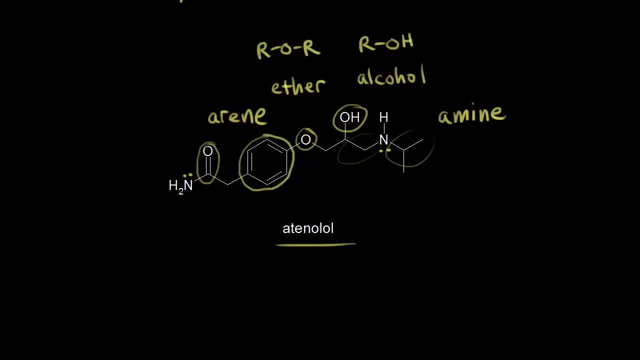 an amine. It's an amide or amid. So this is an amide. So a lot of people pronounce this amid, So it's not an amine. So let's talk more about the difference between an amide and an amine. 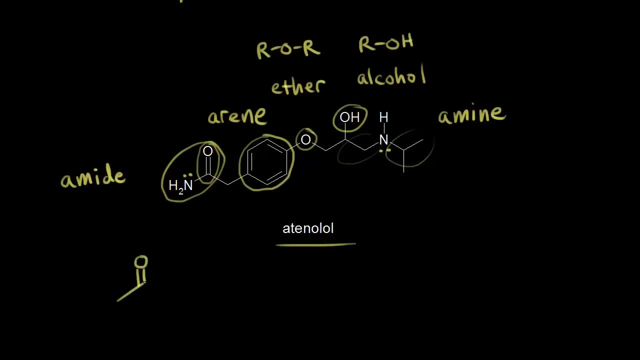 So let me go ahead and draw out another compound here So we can see. we have our NH2.. And then we have our carbonyl. So for this one we have our nitrogen directly bonded to the carbonyl carbon, And that's what makes this an amide. 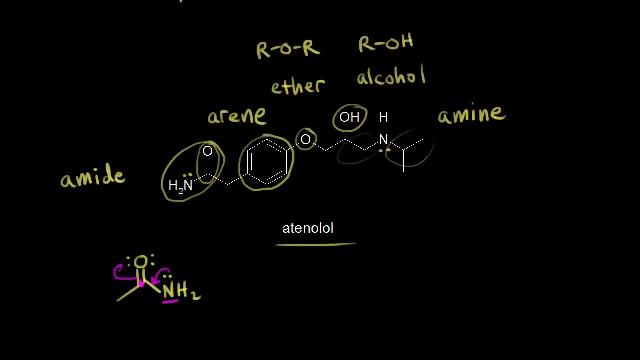 We can move these electrons into here and push these electrons off onto the oxygen, So resonance is possible with this compound. So this is an amide or an amid. If we move the nitrogen further away from the carbonyl, Let's go ahead and 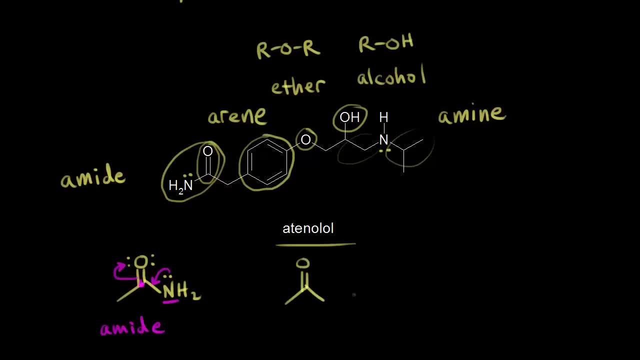 do that over here. So we have our carbonyl, And now our nitrogen is further away. Now we don't have any more resonance. You can't draw a resonance structure showing the delocalization of the lone pair of electrons on the nitrogen. 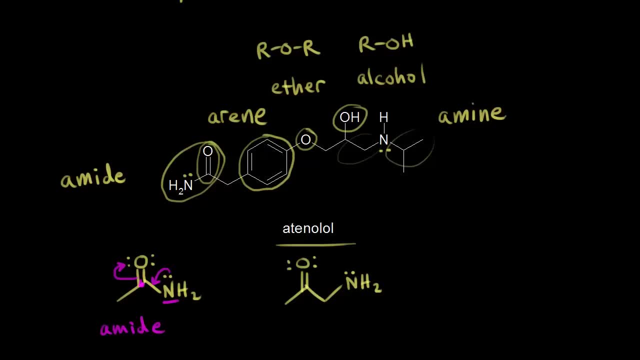 So now we do have an amine. So this over here, this would be an amine. Let me change colors, Let me do blue. This is an amine. And then what would this functional group be? We have a carbonyl. 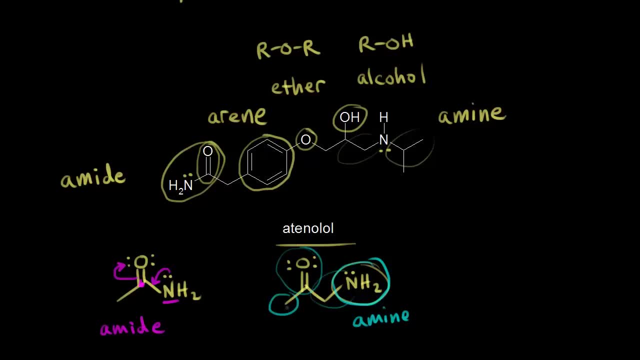 And then we have an R group on one side, R group on the other side. That is a ketone. So this is a ketone and an amine. And then over here we have an amide or an amid. So make sure to know the difference between these. I've seen a lot of